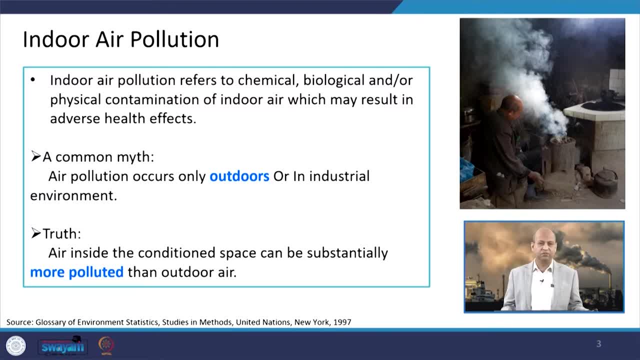 is only outdoor problem or only ambient air related problem, and that may be the reason that you know most of the discussions happen is regarding only ambient air quality. We have so many, you know, standards like national ambient air quality standards, but related to indoor, you know. 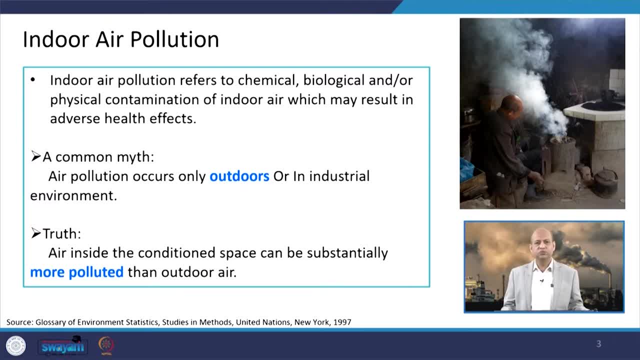 air quality. hardly any standard are there. So there is a huge gap. We think that only in industrial areas or industrial environment or outdoors this air quality may deteriorate and there may be air pollution kind of thing. But fact is that, you know, the air inside the buildings or the micro environments can be highly polluted, and we are 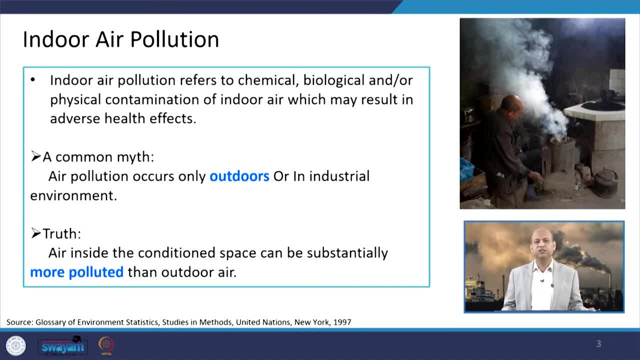 not aware of that. you know several kind of pollutants may be there inside the buildings and we can get exposed to that Sometimes at times. you know the air pollution inside the building is the ambient air and there are certain reasons. we will discuss about those aspects also. 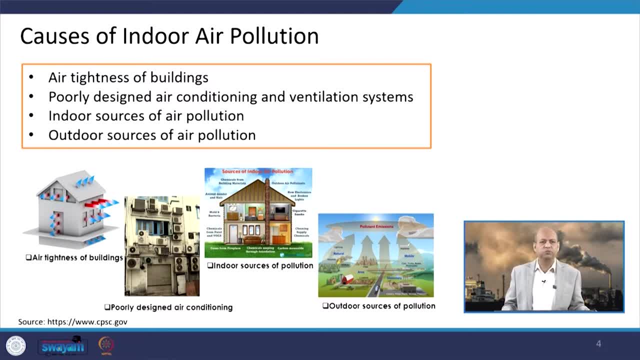 So when we, you know, talk about the causes of indoor air pollution, then we come across like, for example, air tightness of building may be responsible because it prevents the air exchange. Circulation is inhibited, air circulation is inhibited and, whatever you know, emissions. 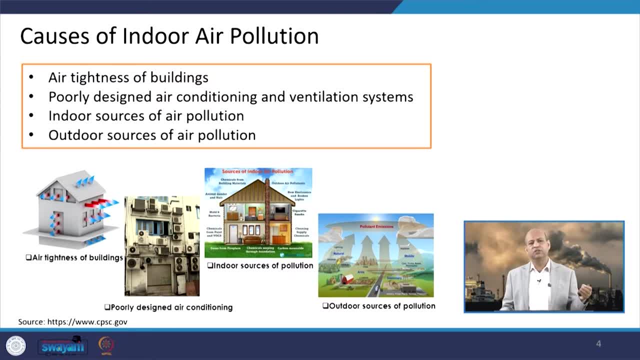 are being generated indoor, like from kitchen or from smoking or any other activity, like from dryers or washing machine or mopping and, you know, brooming, all those kind of activities. they can generate a lot of dust or air pollutants and they may be inside the building because this air tightness of the building may prevent to. 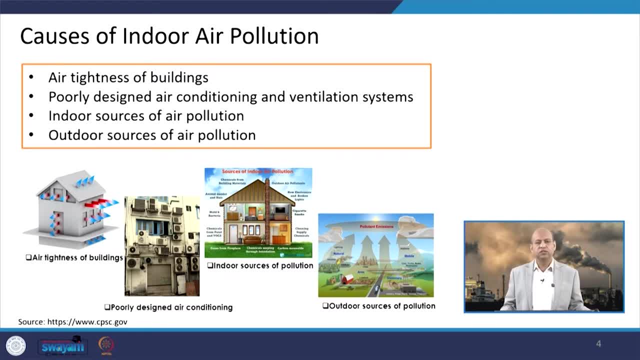 get them out and there may not be proper ventilation. So the poorly designed air conditioning or ventilation systems also adds to the air pollution in the micro environment of buildings. Then indoor sources of air pollution may be there, as I said, like from kitchen or from other. 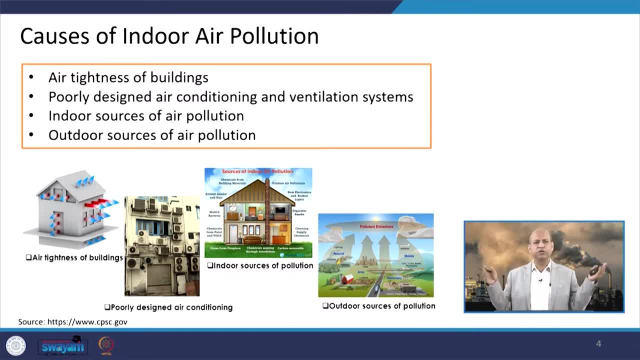 activities we have, even from furniture or from paints, etc. there may be some passive emissions and outdoor sources of the air pollution may also contribute to the indoor environment, because whenever we are opening window or, you know, door, then the air is coming from the outside and then, you know this, inside air goes outside. So if there are significant sources outside, 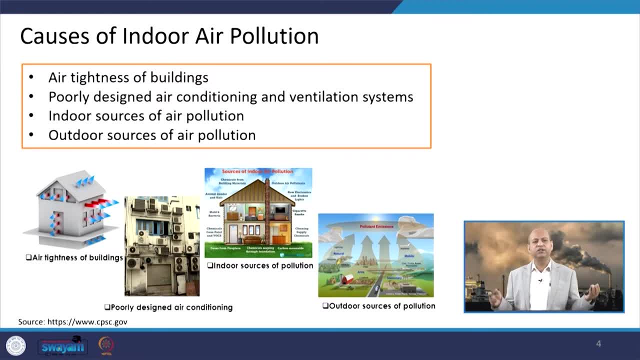 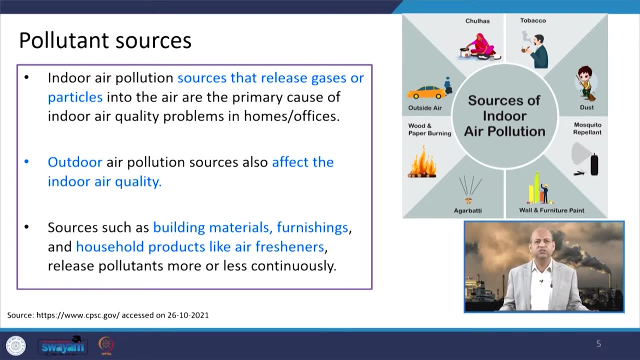 the building and those sources are polluting the ambient air. that air can flush into, you know, rush into the building, inside the building, and that can also add to the indoor air pollution. Well, you know. so when we talk about different sources, basically you know, these are like: 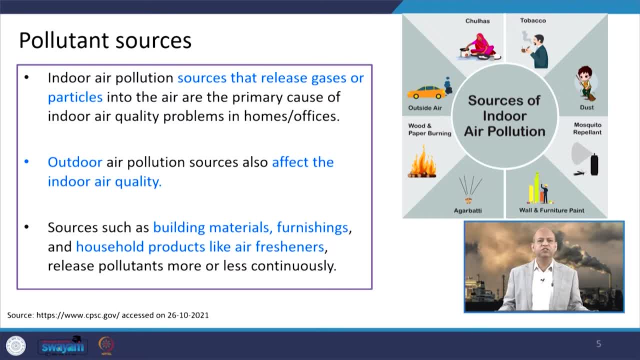 whatever gases or particulate pollution which are coming from- you know indoor air quality problems, from homes or office related activities and, as I said, it can be coming. it can it can come from outdoor activities also, whatever outdoor activities they can add, and you know these chulas or in kitchen, plus tobacco or dust. 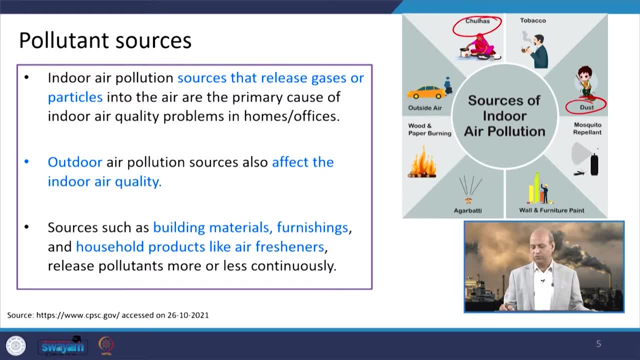 from these kind of activities they may, or even when we are using some, you know, room freshener or these are basically VOCs, volatile organic compounds. they also add into the air pollution inside the buildings. So sources can be several, like building materials or furnishing items or household products like air fresheners, and there are 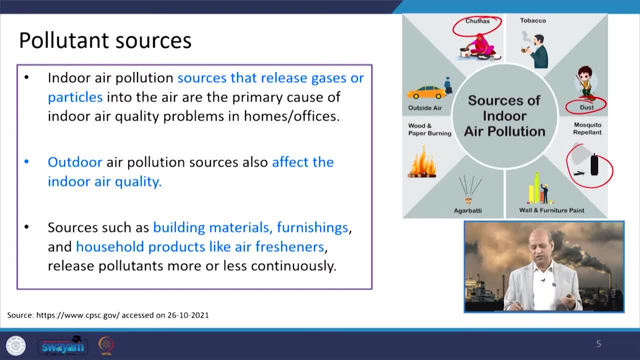 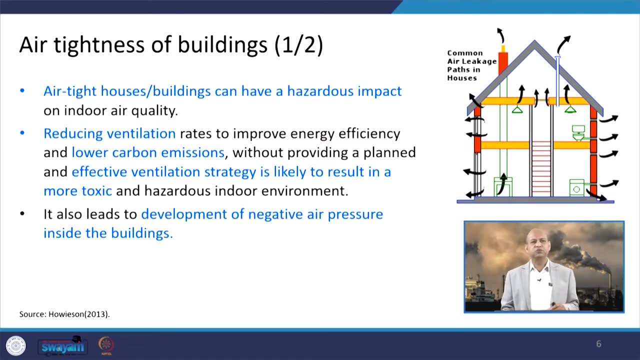 numerous activities which can release, like even when we are doing some sort of you know puja, we are burning something, then whatever things are being burnt that can add into the air pollution inside unless we have proper ventilation system. So when we talk of different aspects, so air tightness of the building is one important aspect. 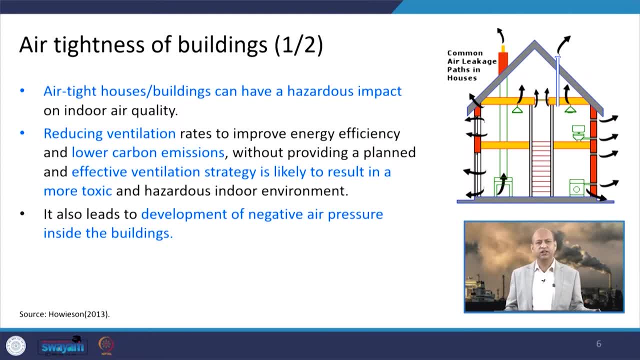 because it prevents, you know, the air exchange, as I said, and it can build up some hazardous impact in the indoor environment as ventilation rates are reduced. sometimes, you know, we feel about like energy efficiency, that we should not go for very high intensity or efficiency of ventilation because then electricity bill will be will be very high. 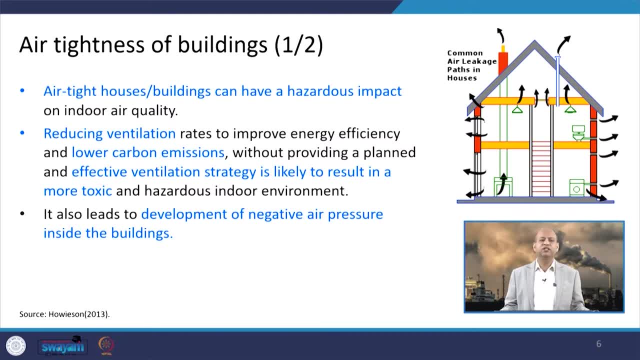 high. So what happens? sometimes people do that this ventilation rate they reduce to improve the energy efficiency and the lower carbon emissions. those could be the reasons to achieve, but then that can result into built up of indoor air pollutants and it can lead to development. 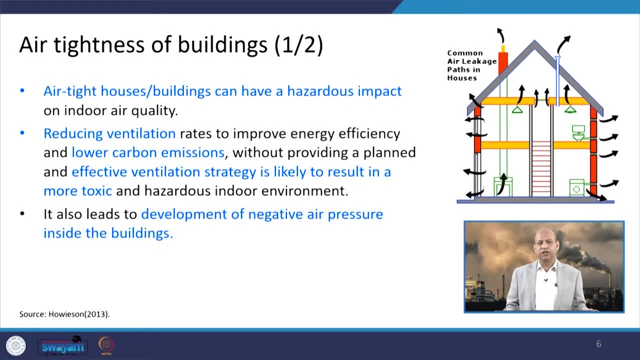 of negative air pressure inside the building. So negative air pressure means low pressure, and if air pressure is outside the building is higher, then again the polluted air can come from outside to inside through cracks, through whatever opening is there, through that air can come, as air is so diluted fluid. 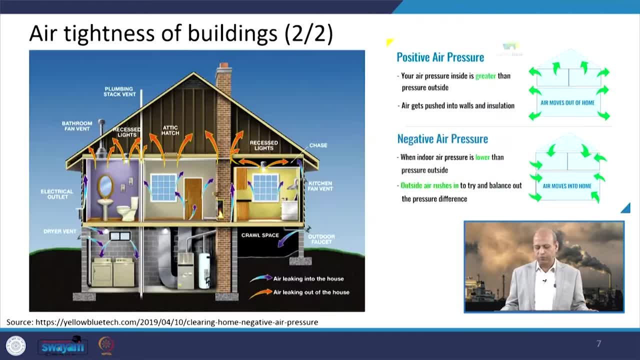 it is very difficult to prevent it to move from one point to another. So you can see here, when it is shown that of course there are ventilation systems, then some positive pressures are there. So if the air pressure is proper and then air goes out in from the inside to outside. 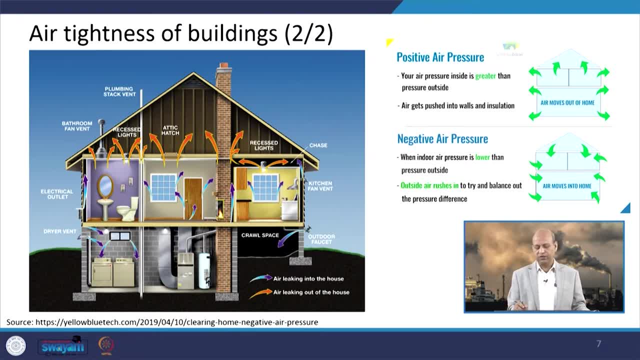 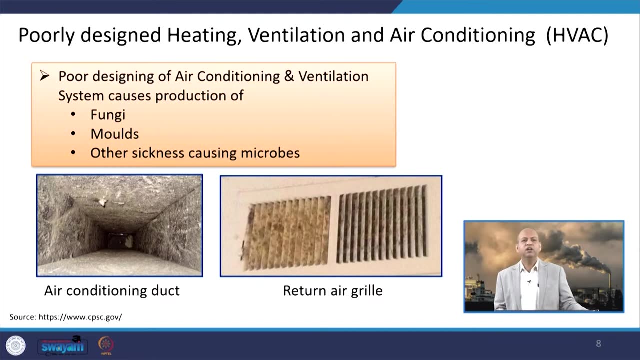 but from outside to inside also. air comes depending upon the pressure. So wherever negative air pressure is there, air will come from outside to inside building. wherever positive pressure is there, air will go out to out from the building to the outdoor environment. Well then, poorly designed heating ventilation and air conditioning. HVAC heating ventilation. 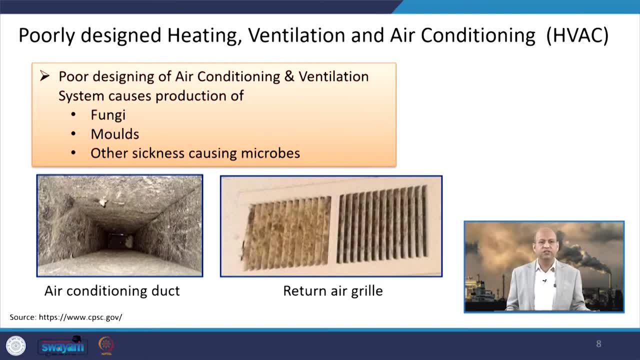 and air conditioning system. If it is not designed properly, then it can also result into several kinds of pollutants, like it can result into fungi or molds or other sickness causing micro microbes or bacteria. all those kinds of things may happen and that can add into allergic related issues. 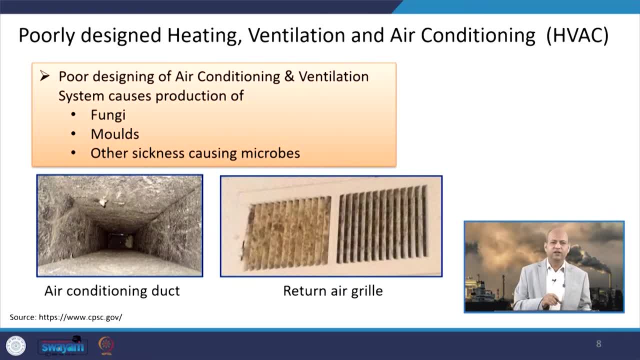 So in air conditioning duct if it is not clean and if it is moist and it can cause microbes related activities, Then it is very dangerous to health issues And return air grill it is. if it is not cleaned regularly, periodically that can also cause that can also get converted into sources of air pollutants rather than air conditioning. 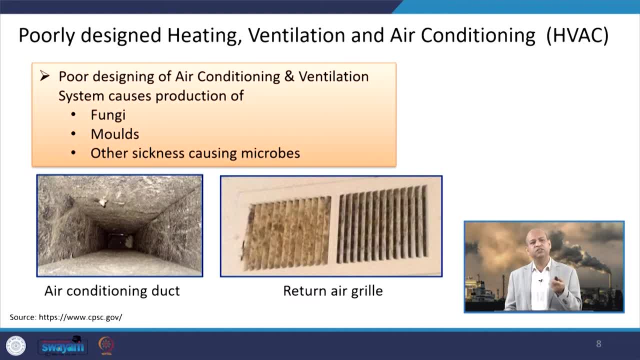 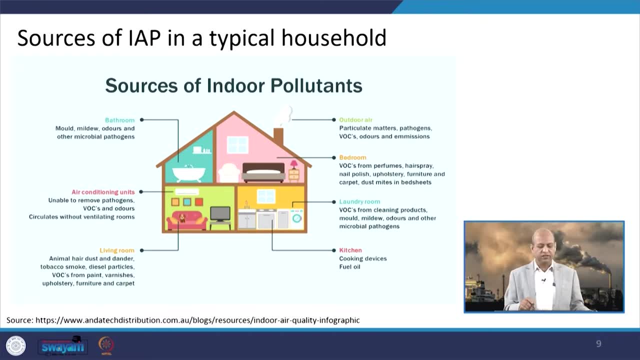 it will. it may reduce the temperature, of course, but it can add to several kinds of air pollutants. So the sources of indoor air pollution in a typical household can be seen in this pictorial representation, For example, like from bedroom can be there bathroom or air conditioning units, living 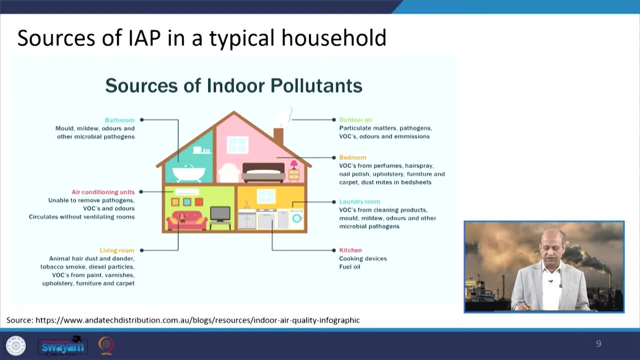 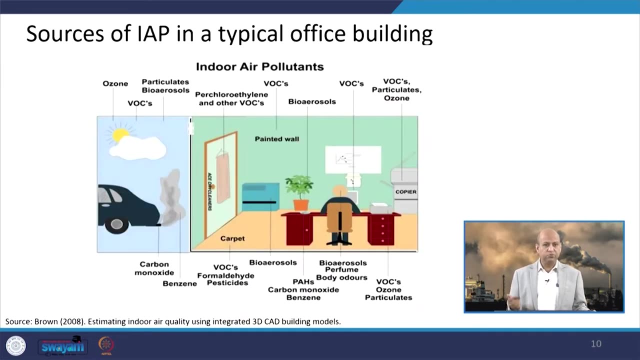 room and laundry room where VOCs can be generated by these detergents, etcetera, those kinds of things, cooking devices, all these kinds of activities can add into one or the other kind of air pollutants inside the building And in office buildings. then there may be additional sources like photocopying machine. 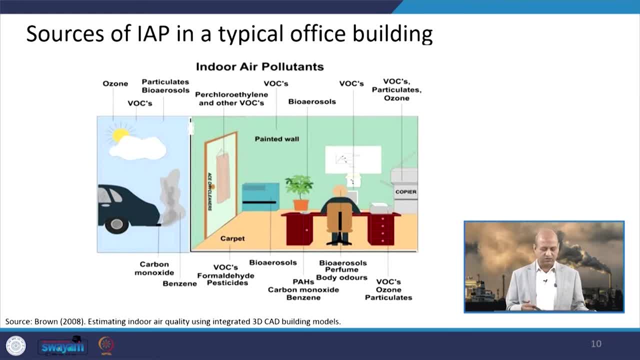 can be there, Okay, Or heaters or some other kind of activities- carpets. carpets capture lot of dust. If we are not doing proper vacuum cleaning then it can be source of lot of dust or particulate matter of fine nature and it is very health hazard. 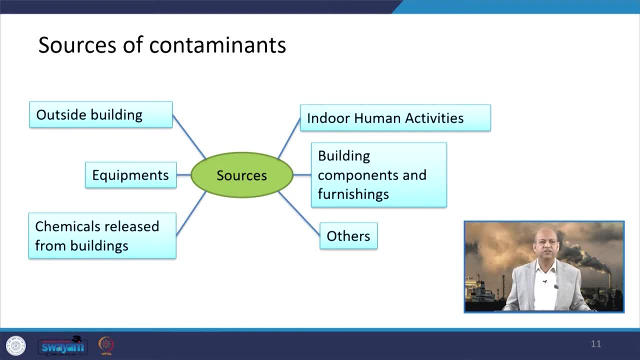 Then if we club them as different kind of sources, then we can say that indoor human activities can add into the air pollution inside the buildings And building components, Components and furnishing like furniture or even walls, paints, etcetera. sofa set. 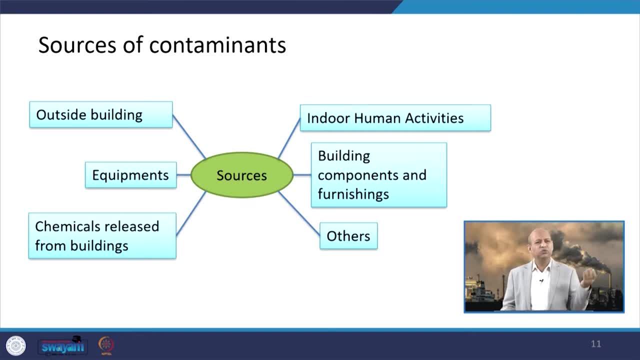 bed set. everything, dust, mites can be there. All those things are of the concern from air pollutant point of view And then from outside building also. as I said, polluted air can come inside. equipments of different nature can add into those. chemicals lead from buildings or when we are using chemicals. 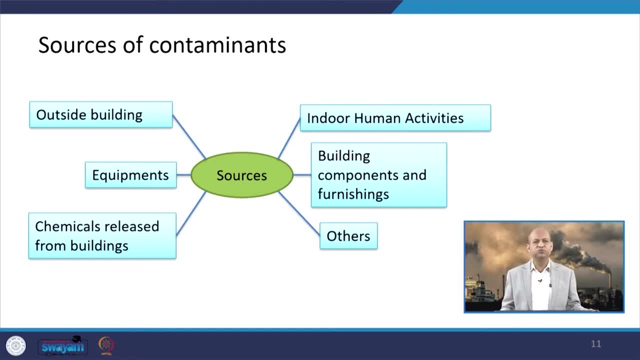 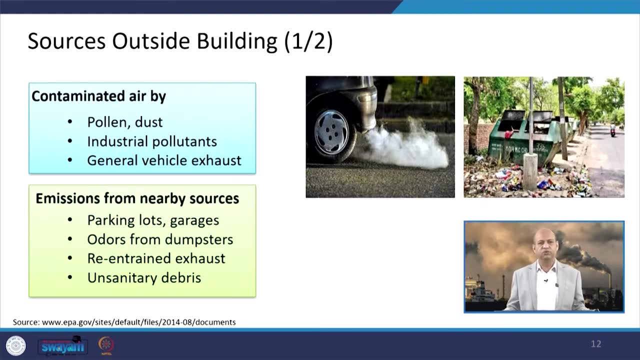 in washroom There are also some fumes, So some fumes may be generated Well, outside the building. there may be additional sources, which are of usual nature as we know, whether it is from industrial stack emissions or pollens from different trees or plants. 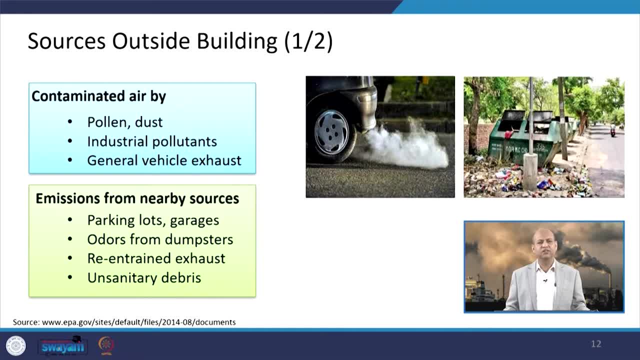 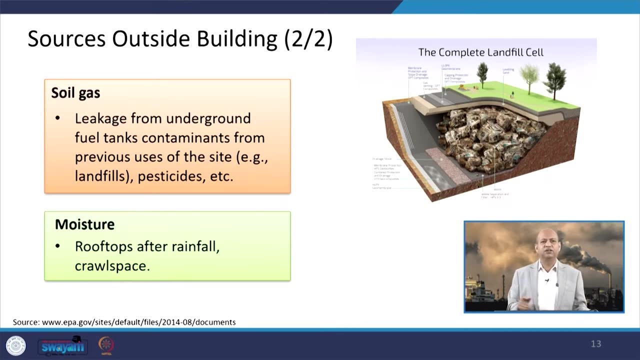 and then general vehicle exhaust- all those kind of things are there from parking lots, garages, orders, from different activities. all those things can be additional sources which can add into indoor air pollution. Then there may be, like these, leakages from underground fuel tanks which have had petrol. 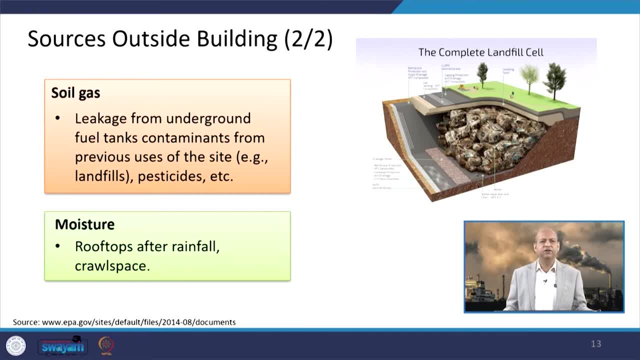 pumps or any other kind of units they can have. And then moisture can also be there, because if proper drainage system is not there within the building, if leakage is there and seepage is there, they can also add into this kind of very fine. 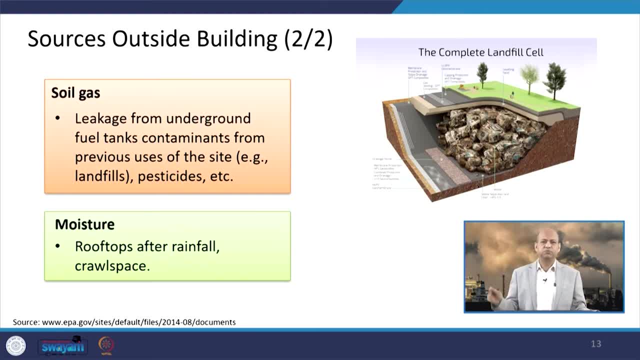 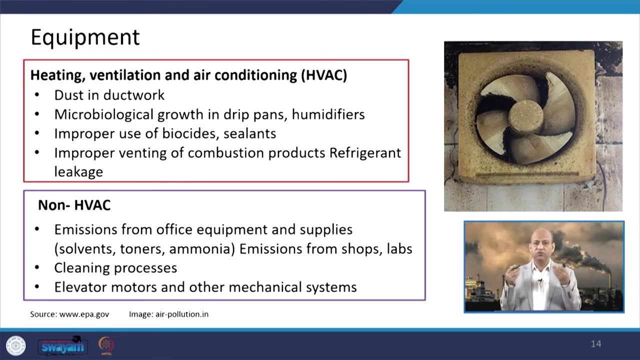 These pollens means pores Pollens, Ok, or those fungi related issues, and they can add into some microbes which are health hazard. basically Equipments as we have: exhaust fan, etc. if we are not cleaning them properly, they can also be like sources of air pollutants. 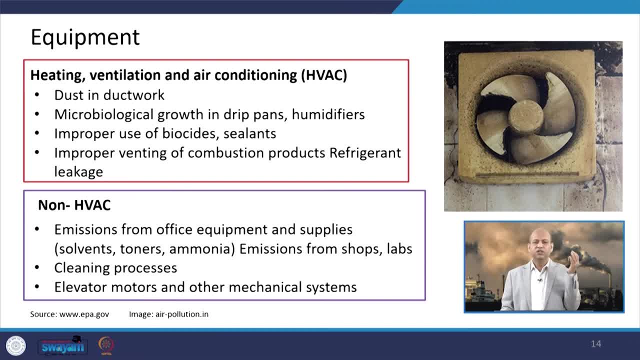 Even those air cleaners. nowadays people use air cleaners or air filters. if we are not cleaning regularly those air filters, rather than cleaning the indoor environment, they can add into air pollution. So it has to be cleaned regularly. So all those kind of equipments: if we are not maintaining them properly, they can add. 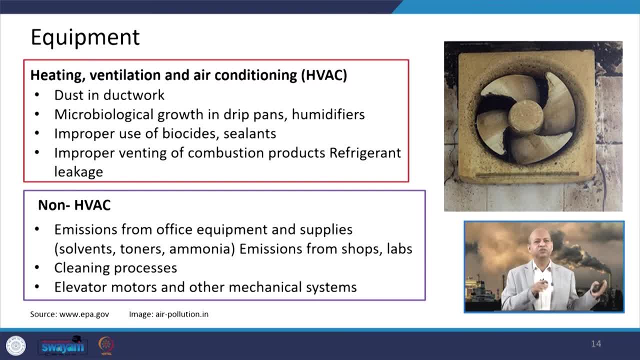 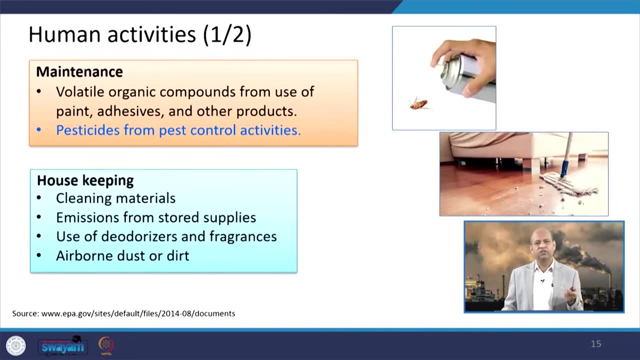 into indoor air pollution. So whether it is heating, ventilation, air conditioning related equipment, or non-HVAC means non-heating ventilation air conditioning equipment, like solvents or toners, all those kind of cleaning processes, all those can emit one or other kind of indoor air pollutants. 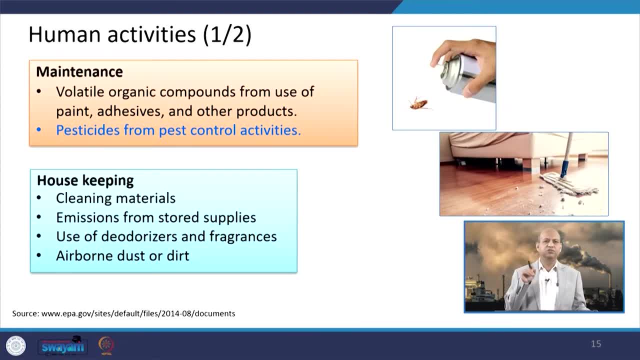 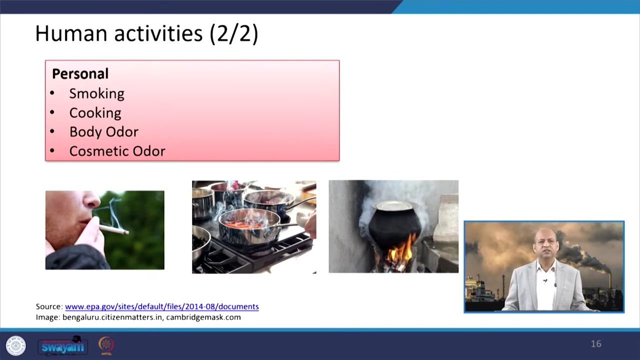 And human activities. as we know, like we are using some pest control related chemicals, pesticides etc. they also add into pollutants inside the building. House activities are there like airborne dust or dirt and then cleaning materials. all those things are there for adding into the air pollution inside the micro environment. 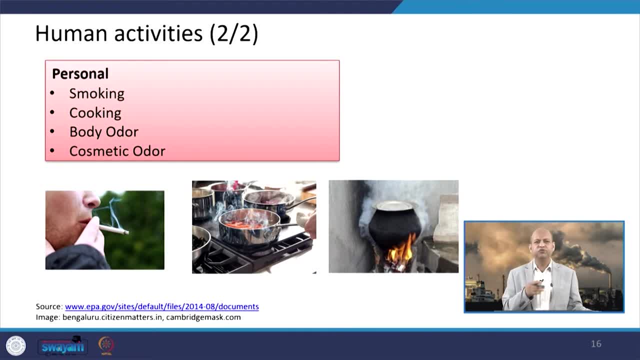 Personal activities like smoking, cooking body odor. If you have any personal activities like smoking, cooking, If we are not clean, then we are also adding into some air pollutants- Our pets. if we are not keeping our pets properly clean, then they can add into several kind. 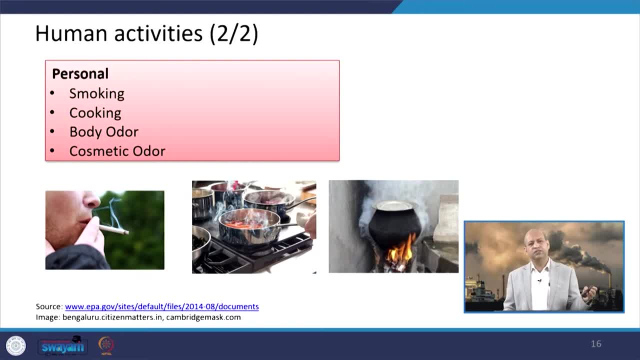 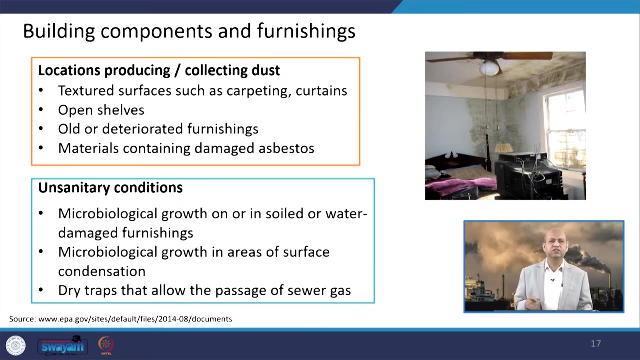 of air pollutants there. hair and many things may be there. Cosmetic odor can be there, all those things. Whatever we are using which smell that is basically adding to the air pollution. Then building components and furnishing, as we discussed, like surfaces or open surfaces. 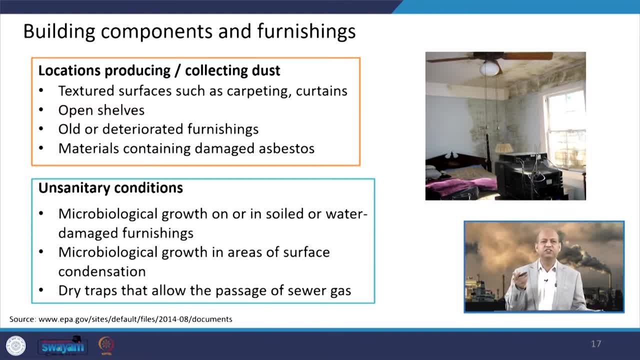 etc. So we are adding some things like materials containing damaged asbestos. all those kind of things are there. Then unsanitary conditions like microbiological growth on soiled or water damaged furnishing. microbiological growth may be there in those surfaces which are moist or and dry traps. 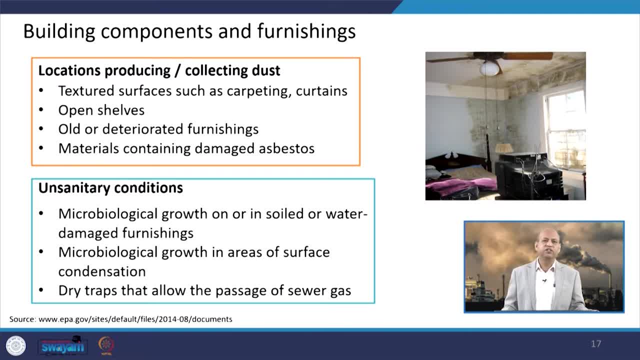 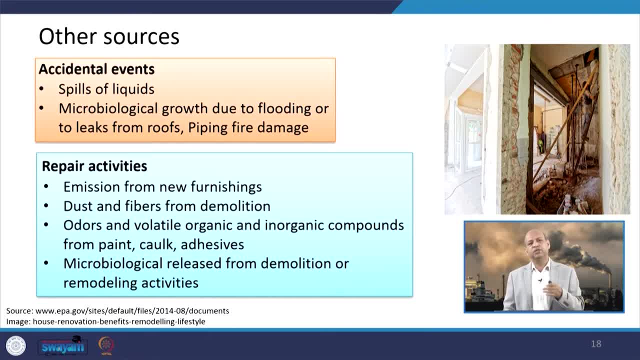 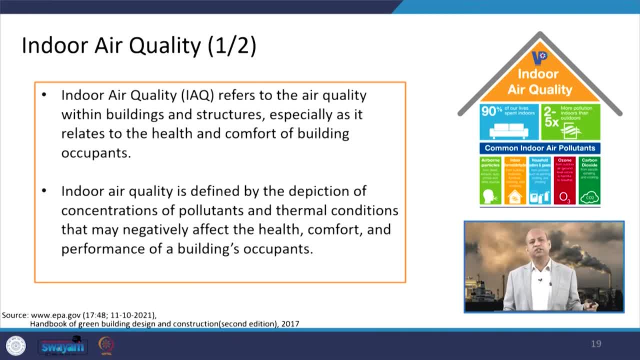 And now we come to indoor air quality, because whatever we have discussed are adding to the indoor air quality. They are leading us to the quality of indoor air. So how do we define what is the indoor air quality? So, theoretically, we can say that it refers to the air quality within the buildings, or 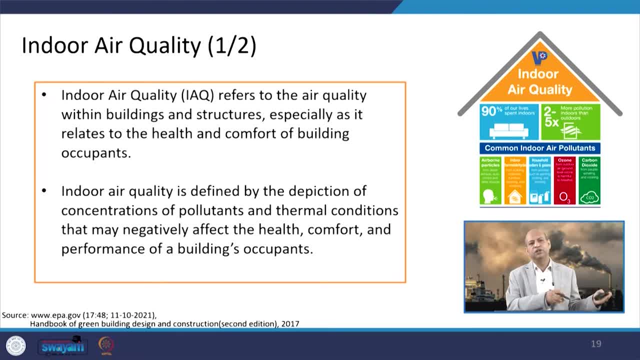 structures, wherever we are living, whether it is a residential building or the office building, especially as it relates to the health and comfort of the building occupants. When your room is properly tight- I mean improperly tight, I would say- and it is not ventilated properly, then lot of suffocation can be there, CO2 buildup may be there and you are not having 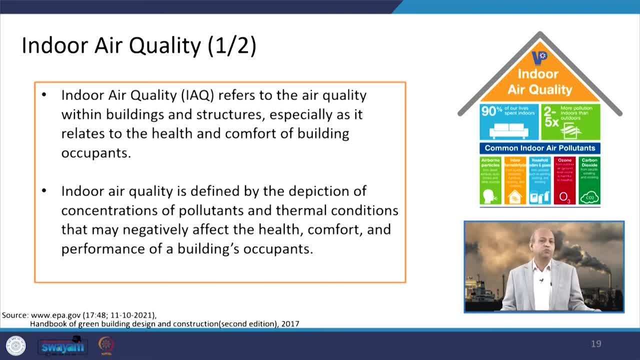 proper oxygen for your air. You are not having proper oxygen to your body and ultimately you may fall sick. So indoor air quality is basically defined by the depiction of concentrations of different pollutants and thermal conditions, plus humidity related issues also And some air pressure. if it is having negative kind of thing, then different air pollutants. 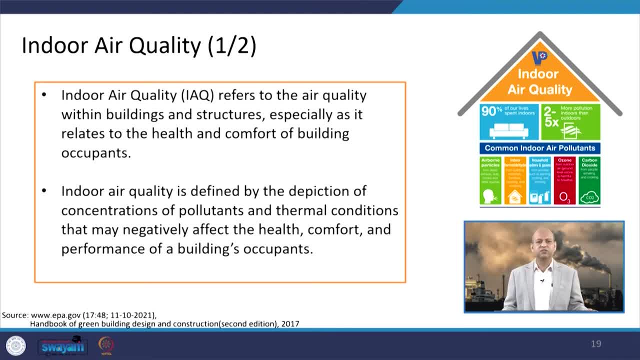 come from outside and they have health impacts of negative nature: discomfort and performance of buildings occupants. occupants can. performance means working performance can reduce, efficiency can reduce. you may fall sick, you may not attend your school or college or office and you have to attend. 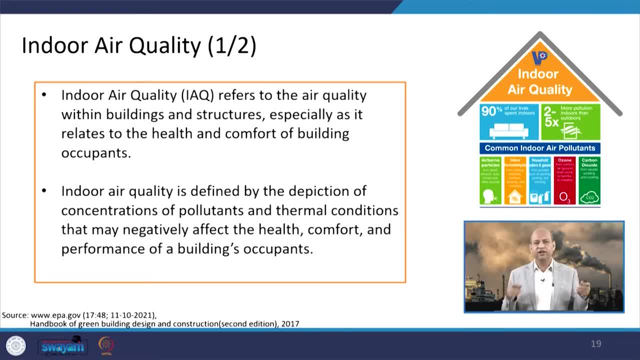 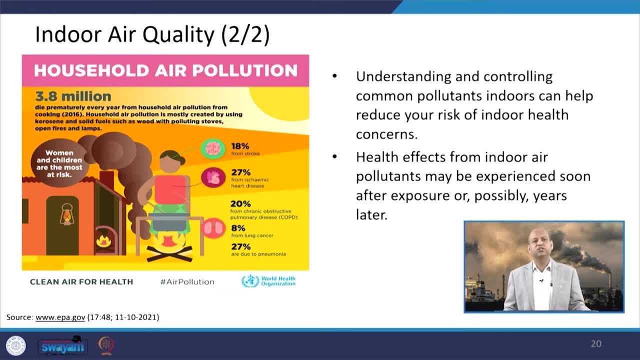 you have to visit the doctor because of some respiratory problems and that may be because of this poor indoor air quality. So, again, as we talk about the, what is the significance of indoor air quality in terms of household air pollution? So, like it is given data: 3.8 million die prematurely every year from household air. 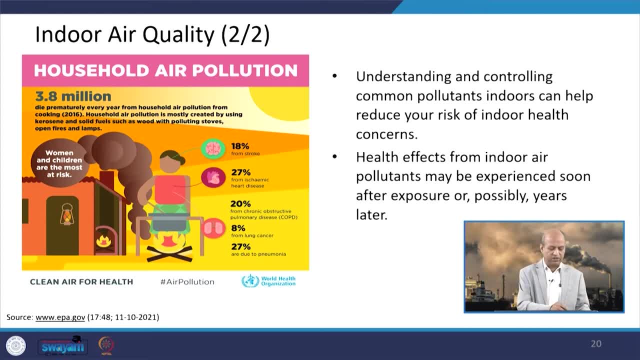 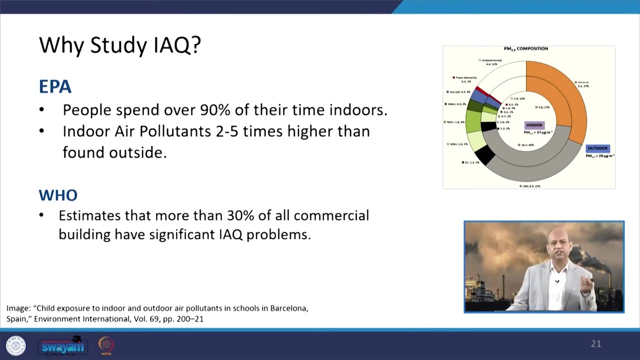 pollution. So from cooking like this is 2016 data, so those kinds of things are there which really alarm that we should be careful about the indoor air quality. So why do we study The reason we know? because it is affecting our health and Environmental Protection Agency. 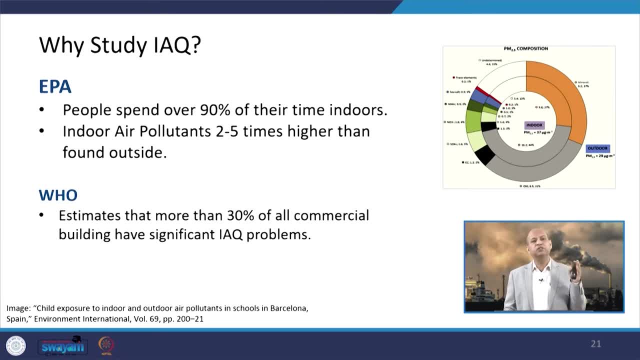 has given some data. like People spend over a year. They spend over 90 percent of their time indoors nowadays and if you look at this, corona means the whole world. almost everyone was inside the their houses. their outdoor activities was restricted very severely. 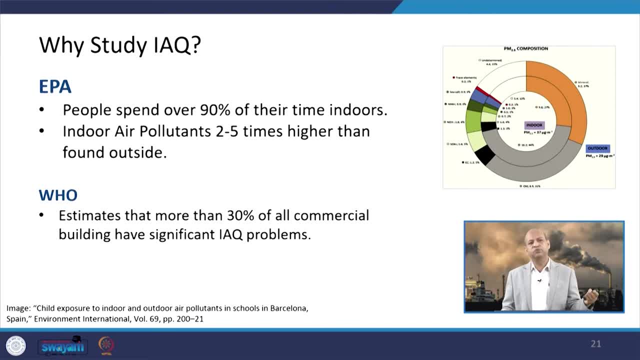 So even this lifestyle is becoming of, so that most of the people, whether they are working in factories or in offices, so they are working in some indoor environment And the air pollutants in those micro environments are two to five times higher than the outside. that has been observed. because of those observations, 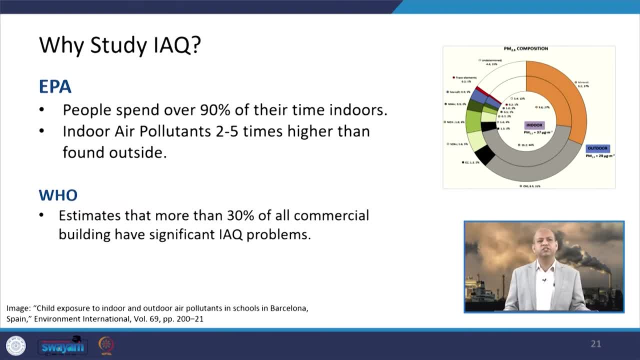 These are the data. World Health Organization also has estimated that more than 30 percent of all commercial buildings have significant indoor air quality problems. So that means the severity of this indoor air quality is affecting lot of people, lot of population, and we should worry about it. 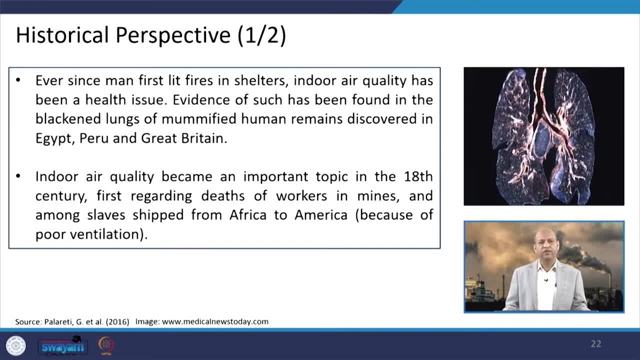 We should be careful, We should do something to improve the indoor air quality. Now, if you talk about historical perspective- whether in past those centuries this was the issue or not- So when we go about the literature, then we find that ever since men first lit the fires, 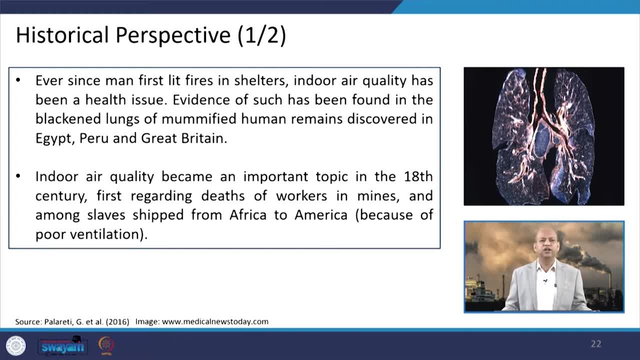 in shelters, in caves. so indoor air quality has been a health issue Basically. there are evidences of such nature that lungs were blackened Because of that particle deposition and it has been seen in this mummified human remains which were discovered in Egypt and Peru and those countries. 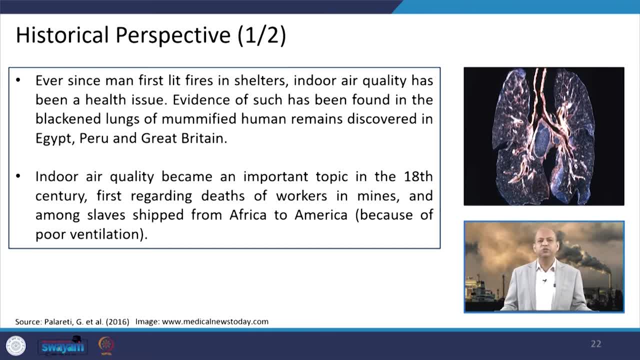 So indoor air quality became an important topic in 18th century very much because of lot of this coal burning and fossil fuel usage And first regarding deaths of workers in mines basically, And those kind of activities, Even this when the slavery was there, so from Africa to America, when ships were filled with 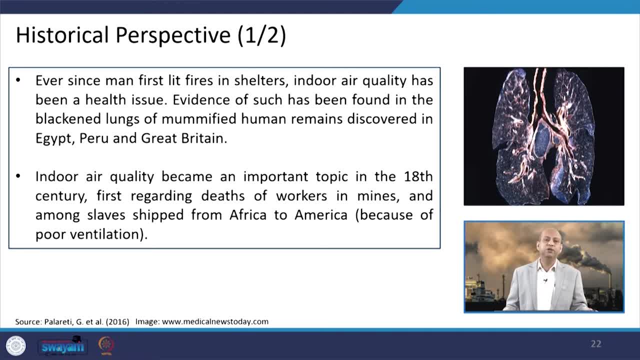 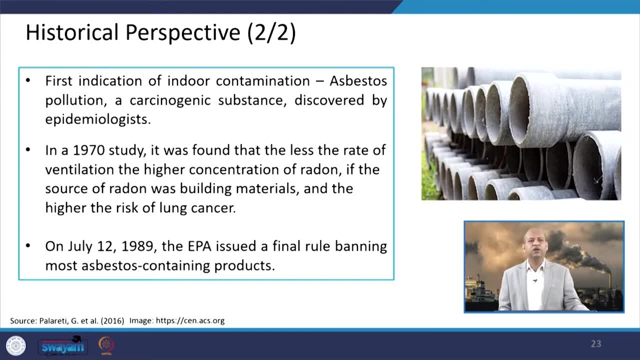 so many people and ventilation was not proper. so many people died and that was basically because of poor air quality. And then we talk about, like this, first indication of indoor contamination in terms of asbestos concentration or asbestos pollution. this is a carcinogenic substance, as you know, and 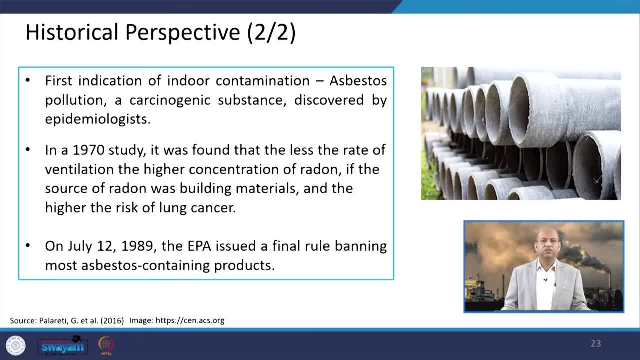 this was discovered by. So in a 1970 study it was found that less rate of ventilation, then higher concentration of radon if source of the radon was building material. And on July 12, 1989 Environmental Protection Agency issued a final rule banning most asbestos. 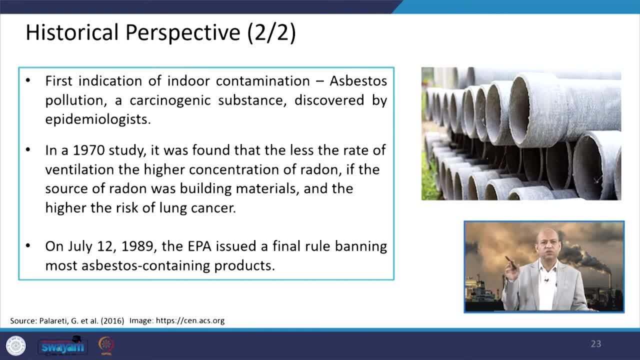 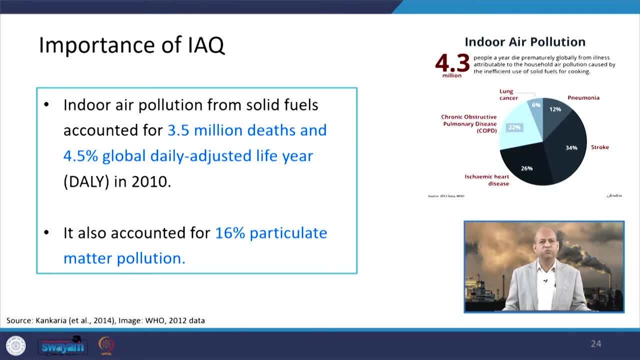 containing products, So those, whatever building material having asbestos. So that was discovered, So that was discarded or banned for usage for the building material purposes. Indoor air pollution, importance of indoor air quality in terms of like from solid fuels when we are using coals, etc. 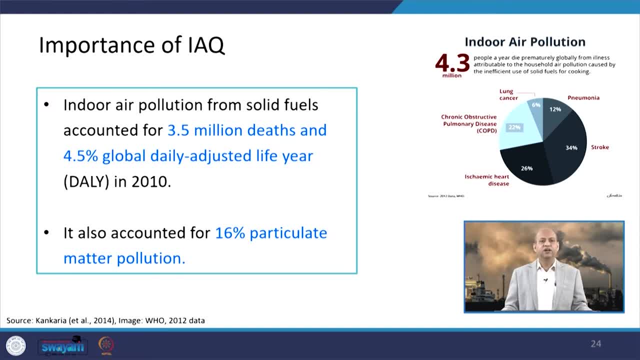 It accounts for 3.5 million deaths and 4.5 percent of global daily adjusted life year. This kind of data are there from a study and it also accounted for 16 percent particulate matter pollution. So that way you know, it is a very significant issue that indoor air quality has to be clean. 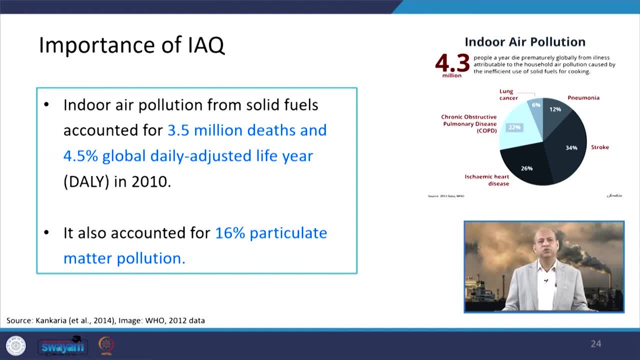 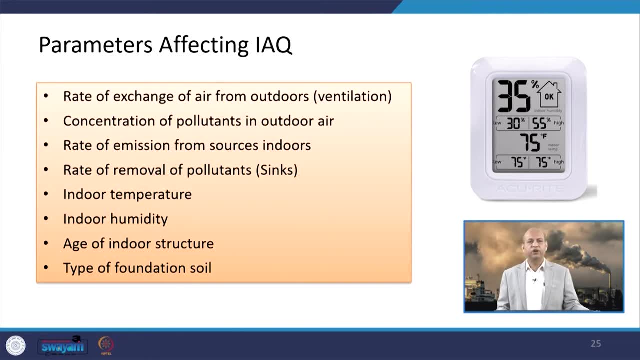 otherwise large number of population can get exposed to its harmful effects. Then what are the parameters which affect or influence the indoor air quality? So, when we list them, like rate of exchange of air from outdoor, like ventilation outdoor to indoor, what is the air mass exchange which many mechanical engineers usually read about? 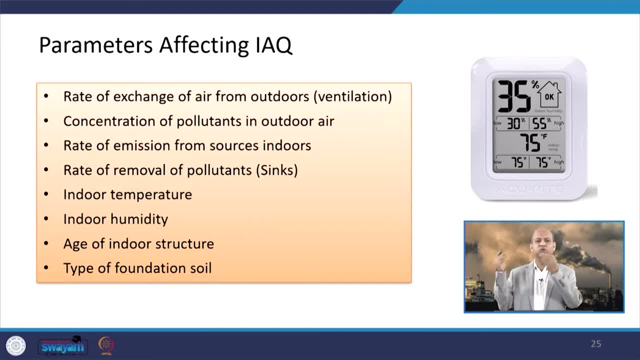 study about And the concentration. So the concentration of pollutants in the outdoor air, rate of emissions from sources. indoors, rate of removal of pollutants like sinks. are there some? indoor temperature, indoor humidity, age of the indoor structures or building material, type of foundation soil. 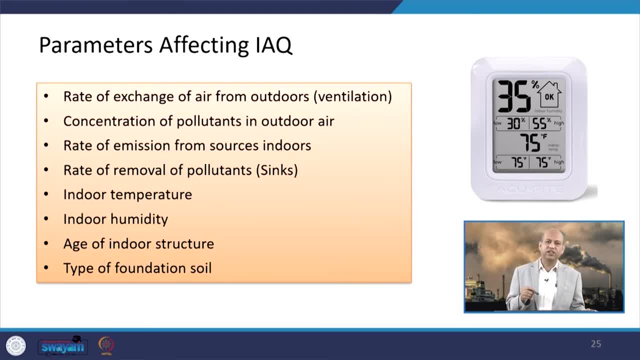 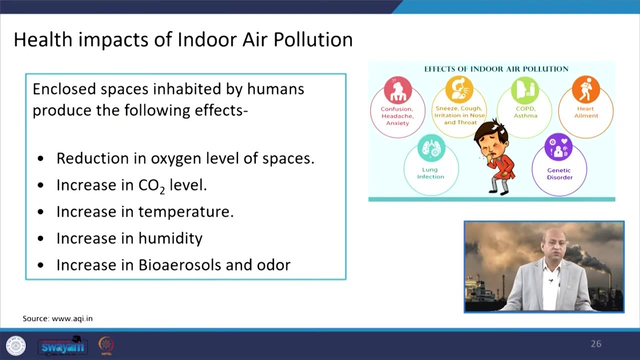 because if it is contaminated, like suppose it was a landfill site and you have constructed buildings there, So maybe some very harmful chemicals are there and you know, slowly they come out of the soil And they fill up, you know, complete the building atmosphere and you never know this can happen. 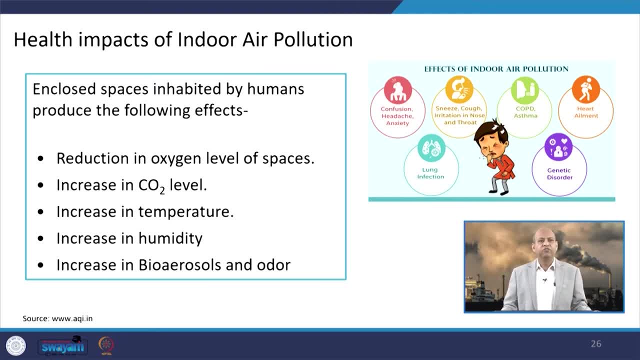 and later on we find that certain health issues are there When health impacts of indoor air pollution are discussed. so you know, the reduction in oxygen level of spaces are the reasons. those are the reasons, like increase in CO2 level, as I said, when you feel suffocated because CO2, you know, increases in lot of quantity. 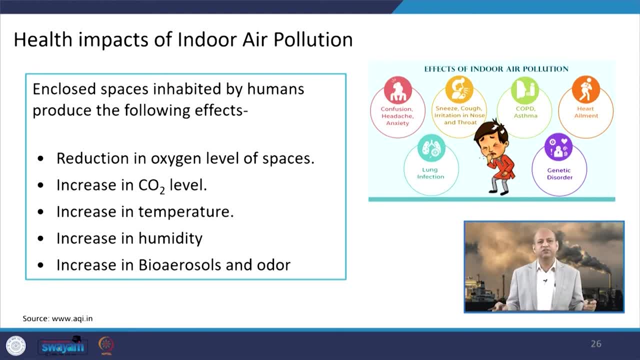 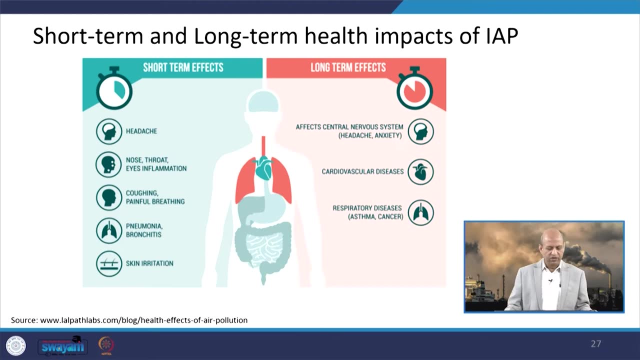 Then temperature may also increase because of certain activities. So that is the reason: Increase in humidity can also add into discomfort, Increase in bio aerosols and odour, that can also affect our daily life. Well, when we talk about short term and long term health impact of indoor air pollution. 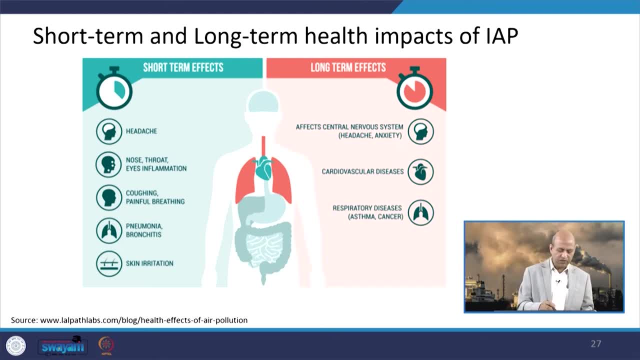 so short term, like it can cause headache or it can, you know, cause some irritation to nose, throat infection, eye inflammation, coughing and painful breathing, those kind of issues. You know now in winter, you know many people They will have these issues and you know, pneumonia or skin irritation, all those things can be. 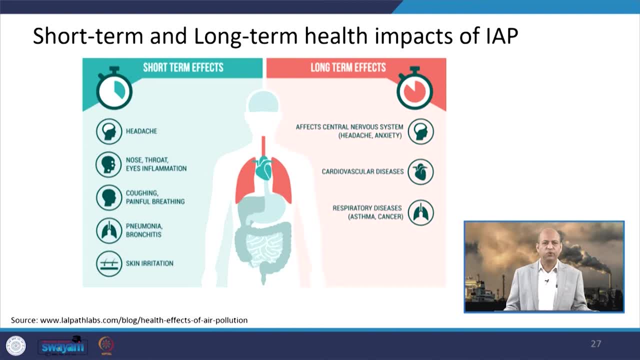 in term. short term kind of effect are there because of polluted air inside the micro environment. When we talk about long term effects, so it can affect, thus, you know, central nervous system, the headache, anxiety all the time. Cardiovascular diseases can also be there. heart related disease can also there. 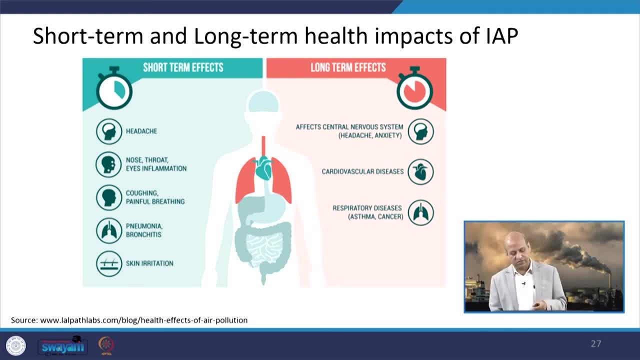 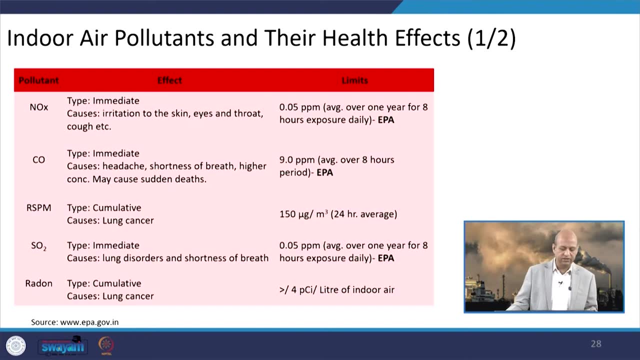 Then respiratory diseases like asthmatic problems may occur Or even cancer causing things can also be there because of constant exposure to the polluted air inside the buildings. When we talk about the pollutant specific effects, their health effects, whether it is outside the building or inside the building it is the same. like knocks is causing irritation. 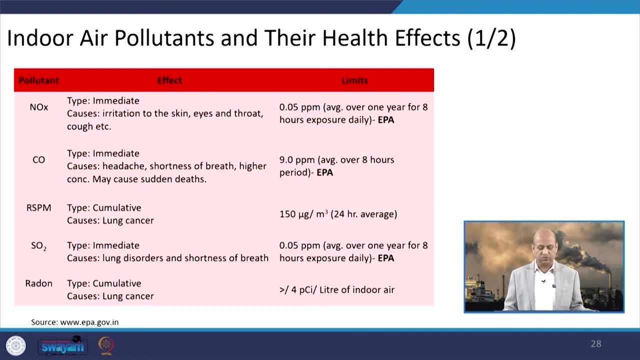 to the skin or eyes and the throat and it can cause coughing also And there are some, you know, limits are given there by Environmental Protection Agency. Some standards are there. This should not exceed These are the limits. CO is having like headache even. in fact CO, as you know, it can cause death also if high. 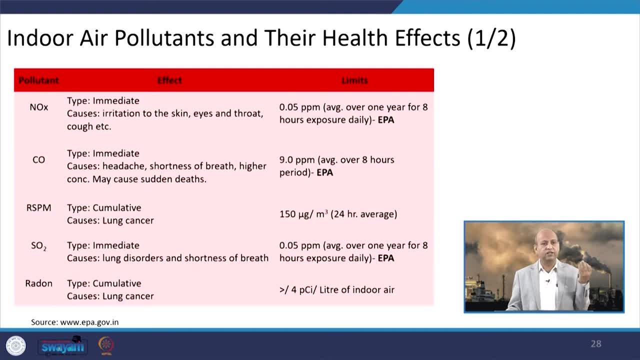 concentration of CO is inhaled and we do not get aware of it because it does not smell or this is odorless, colorless RSPM. respirate this respirable suspended particulate matter, that is PM10. that can cause cancer also. 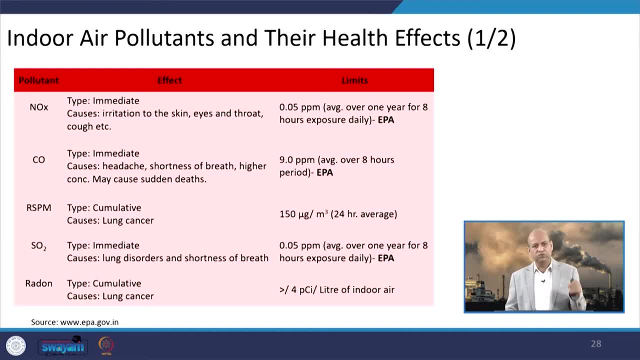 If carcinogenic elements are, you know, correlated. So these are the limits. Thank you very much, Thanks, Thanks, Thank you, Thank you. So you know at least one thing. I would like to share any of the things that were noted. 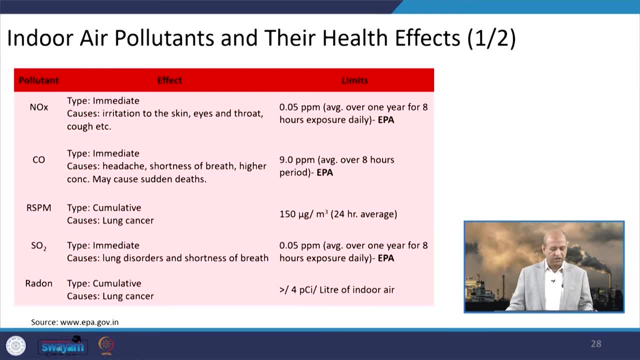 in those particulate matter. whether it is PM2.5 or those fine particles they can enter into our system. SO2 means sulphur dioxide. can result into lung disorder or shortness of the breath. those kind of things may be there And this radon can cause lung cancer. 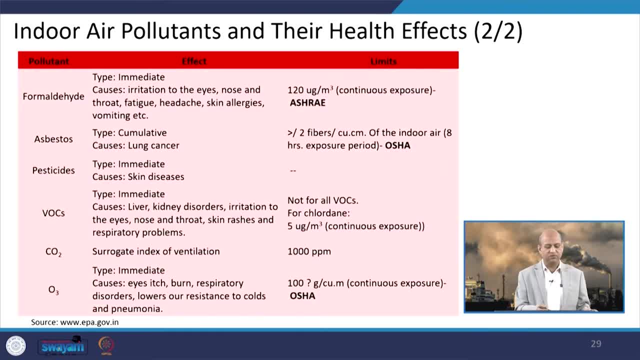 Similarly there are like formaldehyde, asbestos. all these are very health effects can be there. like formaldehyde can skin allergies can result from that. asbestos can cause lung cancer. pesticides- again they are, can result in skin diseases. VOCs: they can have eye irritation or skin rashes. CO2. 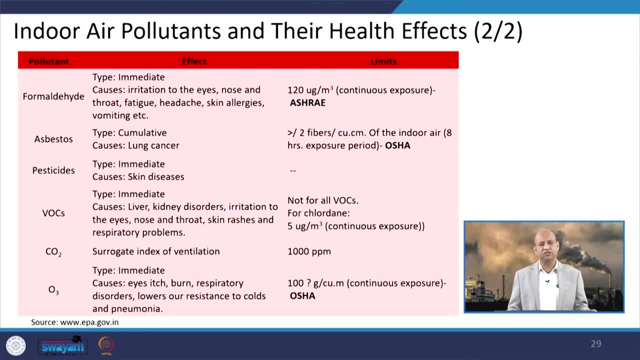 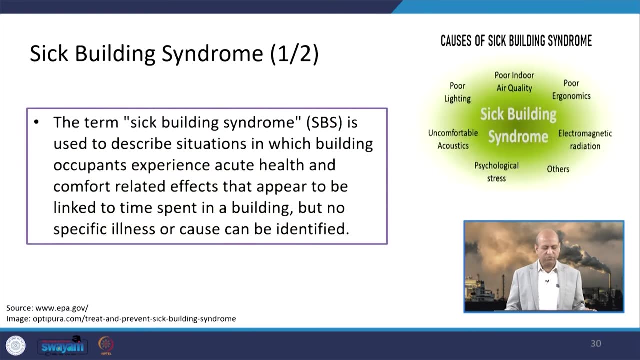 well surrogate index of ventilation, because CO2 is more than ventilation is not good And when CO2 is more and oxygen is less than you feel uncomfortable ozone. many times we have discussed that. it is very problematic and it can cause several kind of problems. 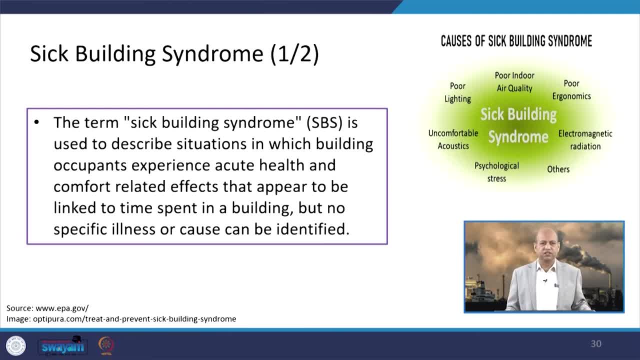 When, then, we come to sick building syndrome? you might have heard this terminology. sometimes you might heard: like some building is blamed, like if somebody goes and the family goes there, they always fall sick. Sometimes we mark a building: this is a bad building. all those kind of things are there. 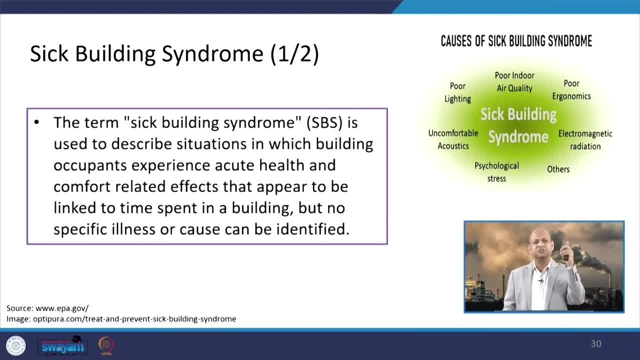 sometimes that do not live in that particular building. it is cursed Anybody has to live in that particular building. If any family came to this building they fell sick. So basically that may be because of certain these indoor air pollutants also. So that is terminology. sick building syndrome is there. 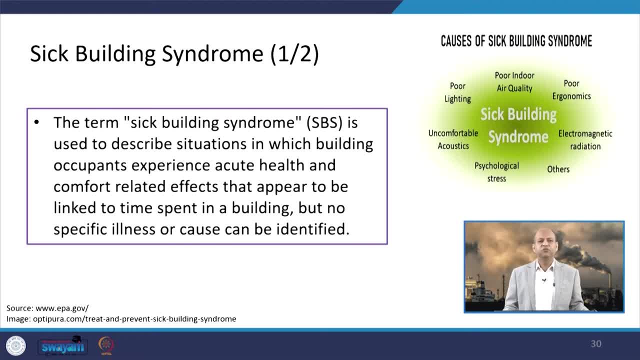 So this term basically is used to describe situation where building occupants experience some acute health related issues. whenever you live in there, then you have breathlessness or some heart related problem or whatever, depending upon what kind of pollutant is there, So specific illnesses may be there. some causes can be identified related to the pollutants. 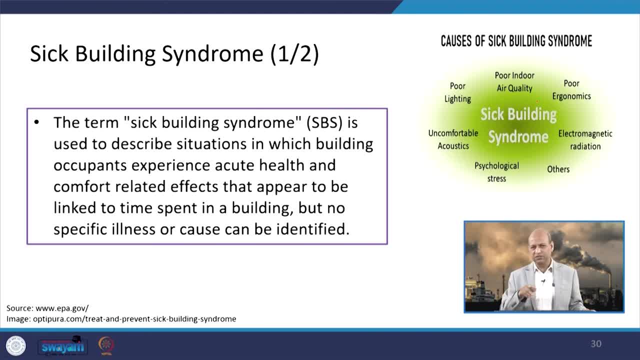 So the poor lighting, poor indoor air quality, poor ergonomics means you can fall if it is not designed properly. and then you can say that this is cursed building. we cannot live healthy here. Uncomfortable acoustics, psychological stress- because if light air, all those combinations. 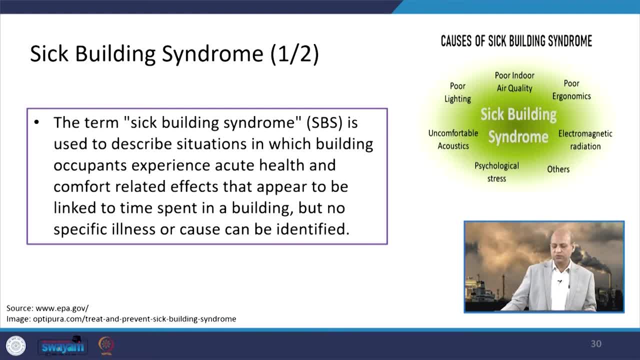 are not proper, then you do not feel good. So those may be the buildings which are known as polluted buildings. Okay, Okay, So those may be the buildings which are known as polluted buildings. So those may be the buildings which are known as polluted buildings or result into sick. 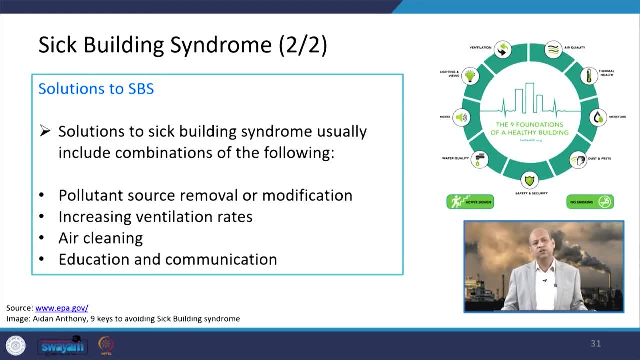 building syndrome. Okay, And the solutions for that, that we should really care about this: lighting, air circulation, all those things So we can solve that problem and the air cleaning, increasing ventilation rates and proper communication with the residents and monitoring of the pollutants and then identifying the sources of those. 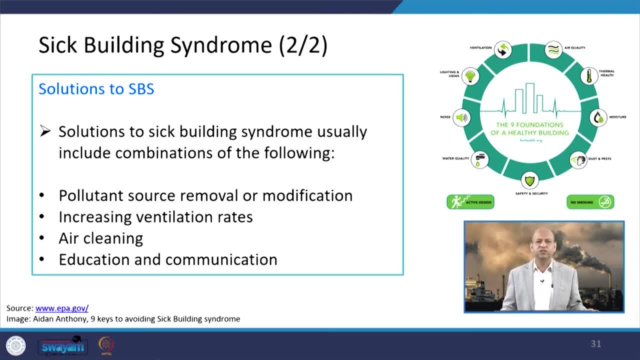 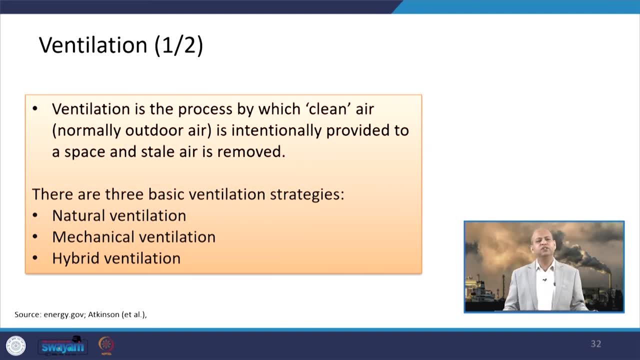 pollutants, removing them, So that kind of thing can be done to make that building as healthy living space. Well, ventilation plays very important role for removing the pollutants from inside to outside And sometimes, as I said, ventilation can even increase the pollutants also, if it is not. 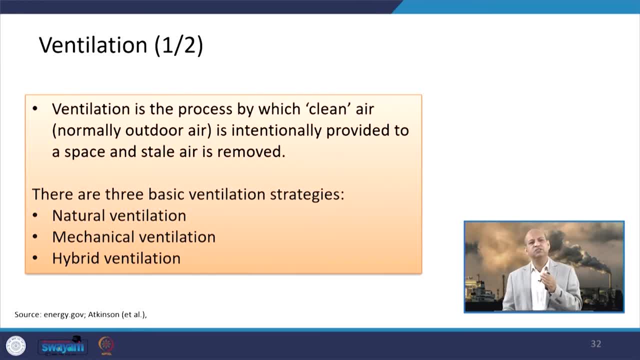 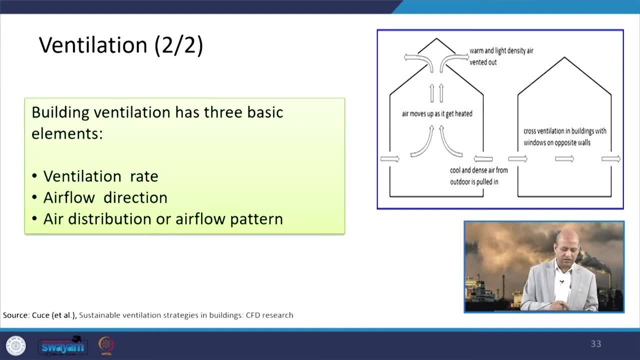 properly designed So there may be natural ventilation, there can be mechanical ventilation or the hybrid system can also be there. So those things can be seen here, like here you see this: ventilation rate, air flow, direction, air distribution, all those things basically play important role, otherwise some corners. 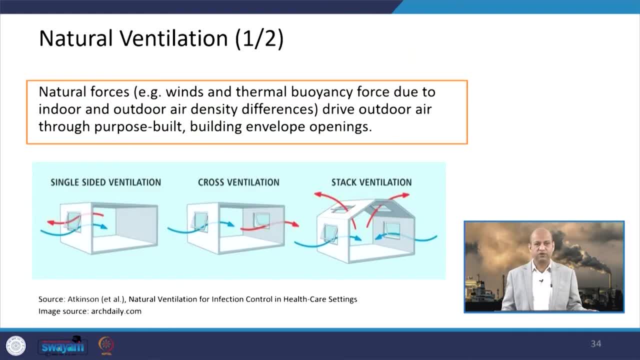 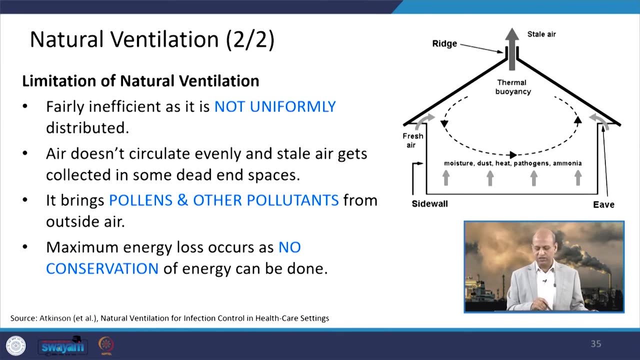 of the building will be highly polluted if ventilation is not proper. Like, if you talk about natural ventilation, it can be in terms of, like, single sided ventilation or cross ventilation, stack ventilation. all those kinds of things can be there And in natural ventilation. basically, you can see here. 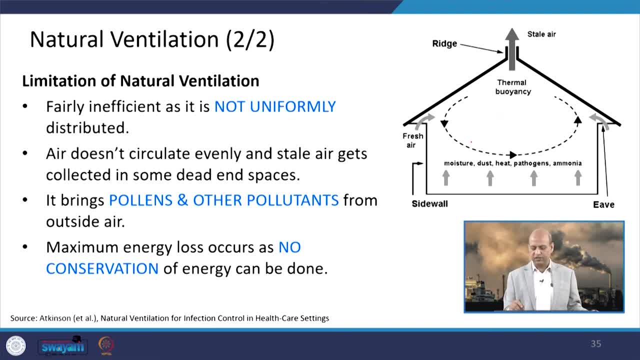 These spaces where circulation happens properly, but it can bring pollens and other pollutants from outside air if it is not properly designed, Because natural ventilation means you allow air from outside to come inside and from inside to outside, with some ventilators which are naturally taking this circulation of the air. 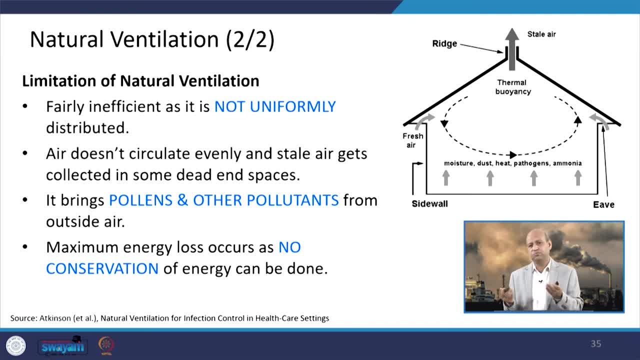 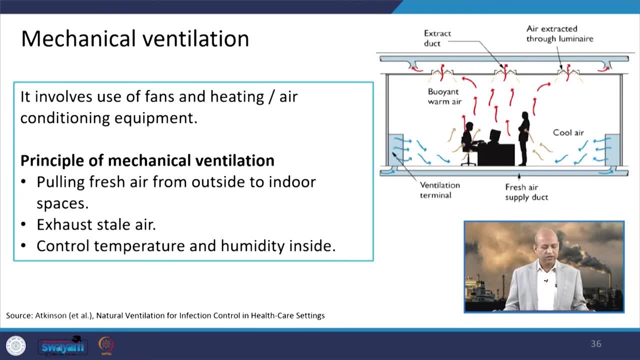 So that way we are not controlling outside air. it is coming just from some openings, So that may be one issue. If it is not clean air outside, then it can be an issue. Mechanical ventilation: basically it can control the air flow, speed, volume, temperature, everything. 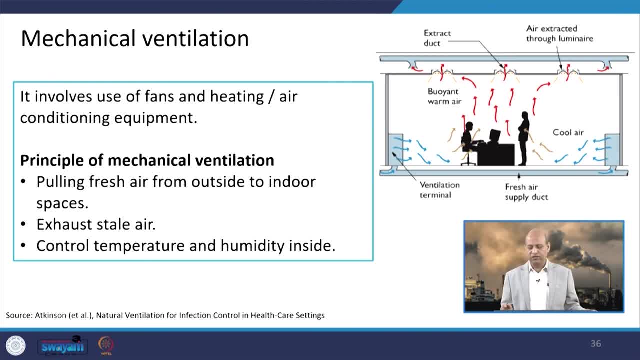 you can control, because mechanically it is designed and that way cool air can come down and then this warm air goes up and it can get out with those particularly systems which are designed for ventilation. So you can see here, like in natural ventilation, There may be some problems. 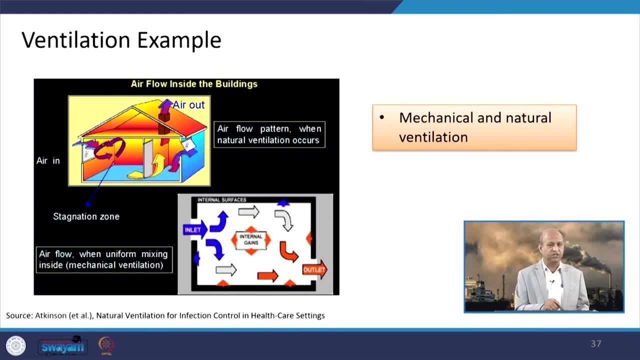 So that may be one issue. There may be some pockets where high level of pollutants may be there because natural ventilation cannot go to each and every corner with uniform flow rate of the air. It has some limitations but mechanically designed proper ventilation system can have. 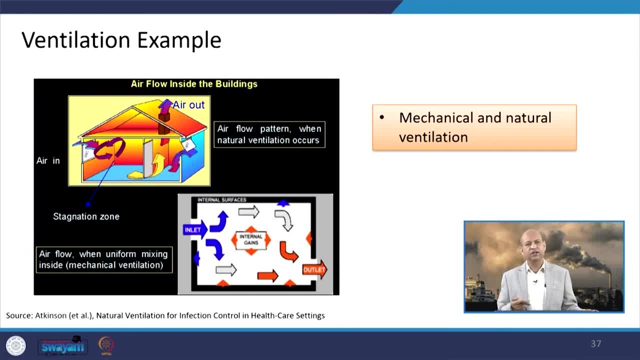 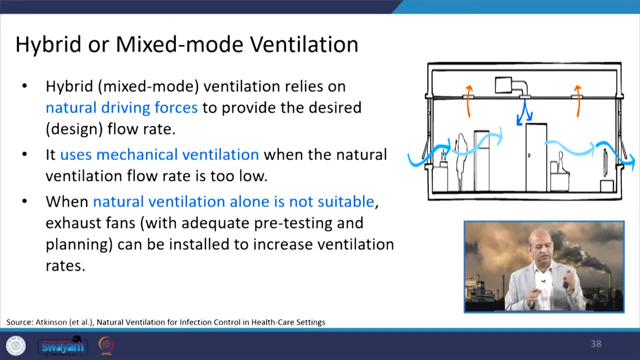 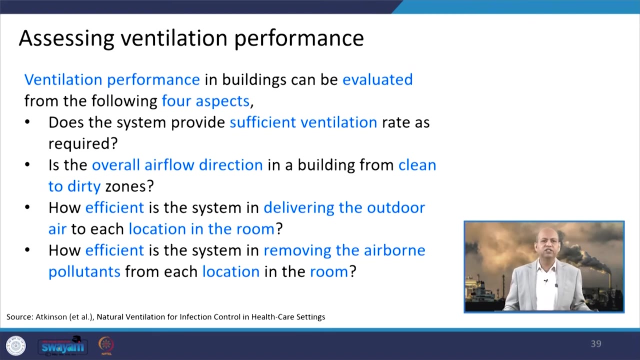 uniform distribution of air circulation and that can remove the pollutants properly. In hybrid or mixed mode ventilation, there are these combined natural driving forces you use And then, whenever this natural pressure difference is not there, then you use the mechanical devices for proper ventilation. When we talk about like assessment of ventilation performance, so we have certain these kind 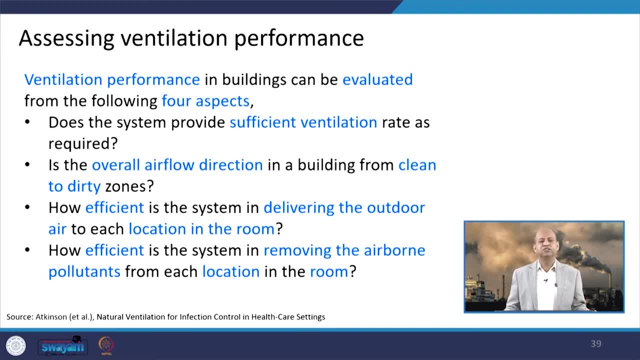 of questions which really help us to see whether the ventilation system is performing properly or not, Like, for example: does this system provide sufficient ventilation rate as required? You can calculate, that Is, the overall air flow direction in a building is perfect. Is the ventilation rate sufficient? 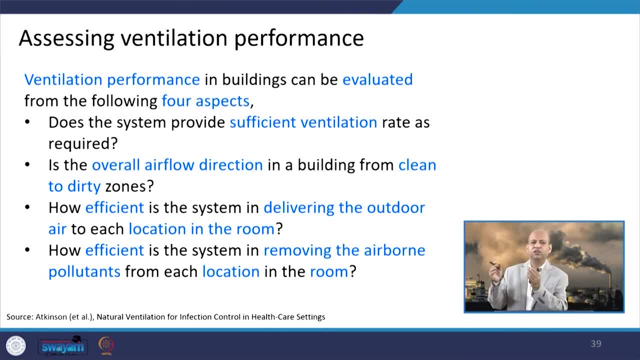 Is the air flow direction correct? Is the ventilation rate sufficient? Is the ventilation rate sufficient? Is the ventilation rate sufficient? And then the next question is: how efficient is the system in delivering the outdoor air to each location in the room And how efficient is the system in removing the airborne pollutants from each location? 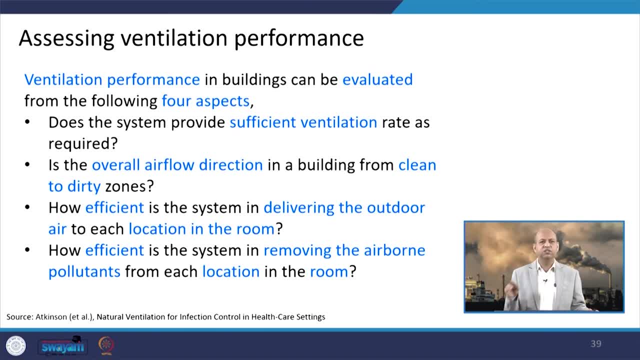 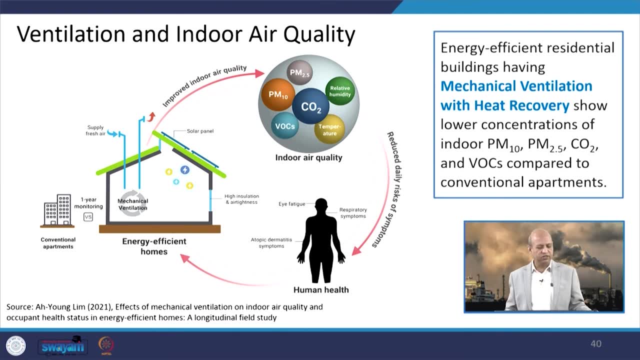 in the room so that room is having clean air. So those kind of things can be seen and for assessment or evaluation of ventilation system. Well, in totality, when we talk about ventilation and indoor air quality, so basically the energy-efficient residential buildings having mechanical ventilations with the heat recovery, they are proved that. 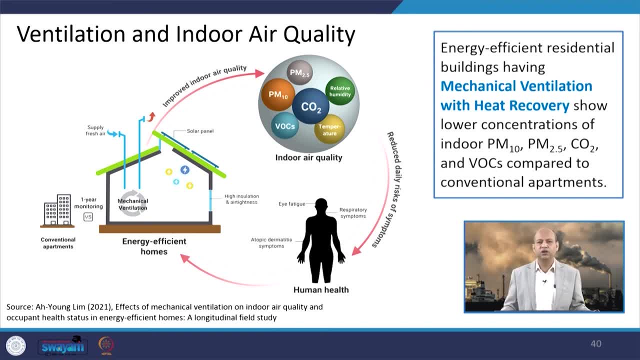 with the lower concentrations of indoor particulate matter, PM10 or PM2.5, carbon dioxide or VOCs, compared to the conventional apartments which do not have the weather properly controlled mechanical ventilation system. So that picture shows that in that proper ventilated system which is controlled mechanically, you can have healthy environment in comparison.